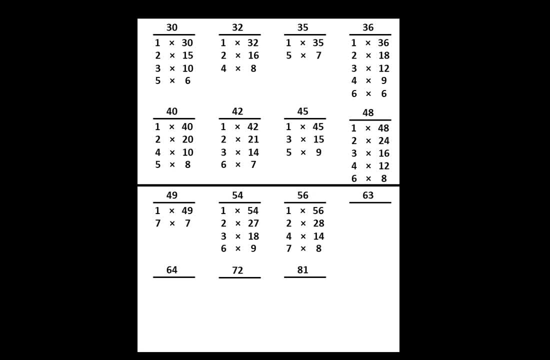 Or 7 times 8.. Those are all the factor pairs of 56.. Let's move to the number 63. On your paper, write that we can think of 63 as 1 times 63. Or 3 times 21.. 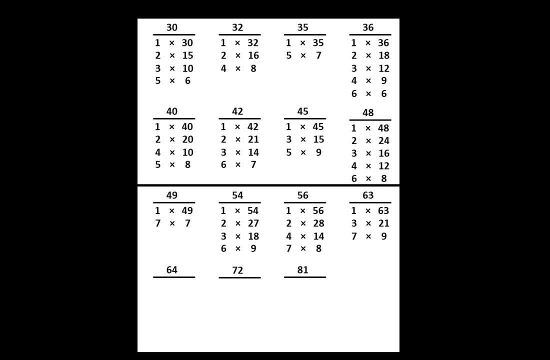 Or 7 times 9.. Those are all the factor pairs of 63.. Let's move to the number 64. On your paper, write that we can think of 64 as 1 times 64. or 2 times 32, or 4 times 16, or 8 times 8.. Those are all the factor pairs of 64.. 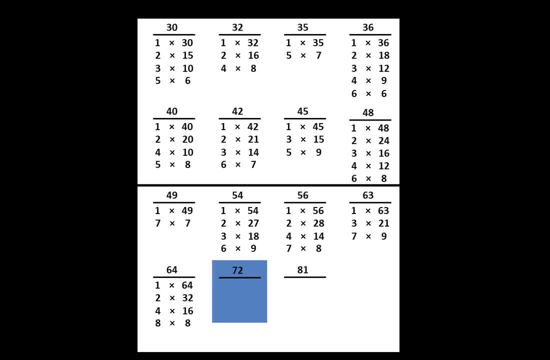 Let's move to the number 72. On your paper, write that we can think of 72 as 1 times 72,, or 2 times 36,, or 3 times 24,, or 4 times 18, or 6 times 12, or 8 times 9.. 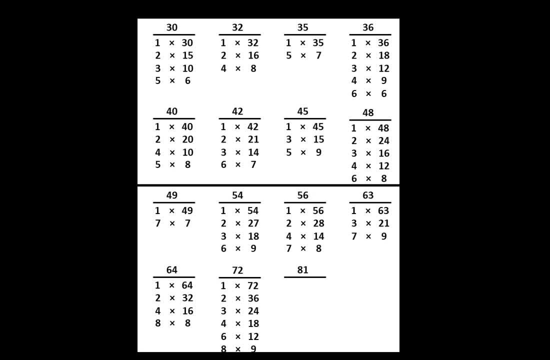 Those are all the factor pairs of 72.. Finally, let's move to the number 72.. On your paper write that we can think of 81 as 1 times 81, or 3 times 27,, or 9 times 9.. 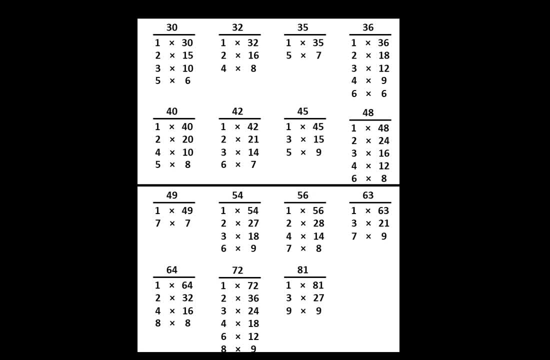 Those are all the factor pairs of 81.. These are all the key factors that we will list. Keep this paper in a place where you can find it easily, because we will use it in future videos. This is the Multiplication Course. My name is Seth.